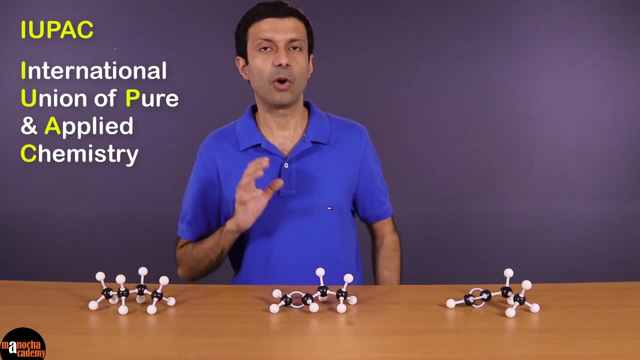 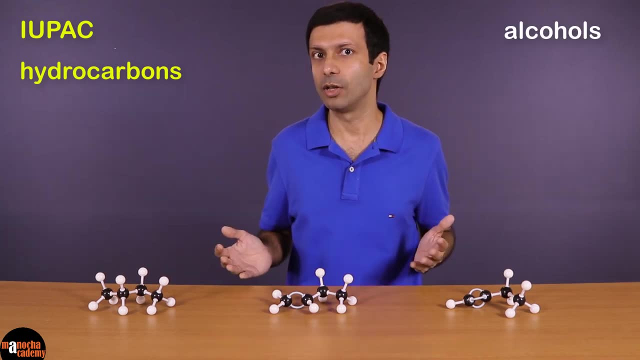 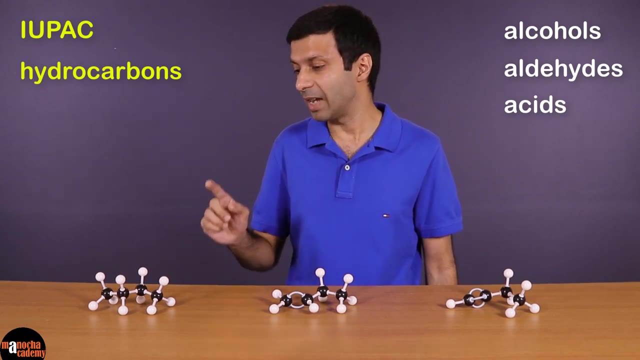 compounds which we are going to discuss Now. we will be discussing only the basic rules for hydrocarbons. The rules for naming compounds such as alcohols, aldehydes acids will be discussed in a separate video. I am going to use this alkane to discuss the basic naming rules for hydrocarbons. 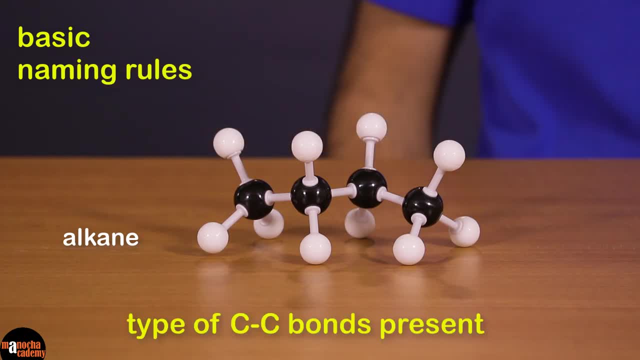 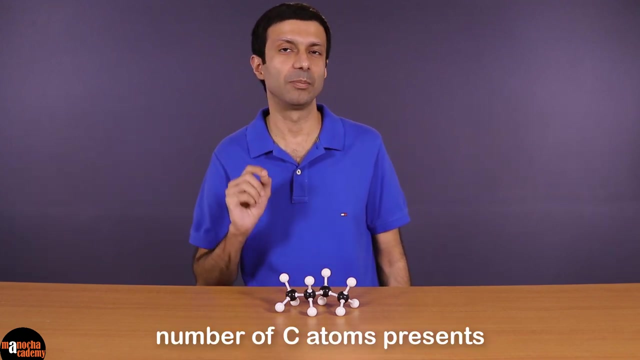 First thing to check is the type of carbon-carbon bonds present. As you can see, we have only single bonds between the carbon atoms, So this is an alkane. The first part of the name depends on the number of carbon atoms present, So we need to count the number of carbon atoms. 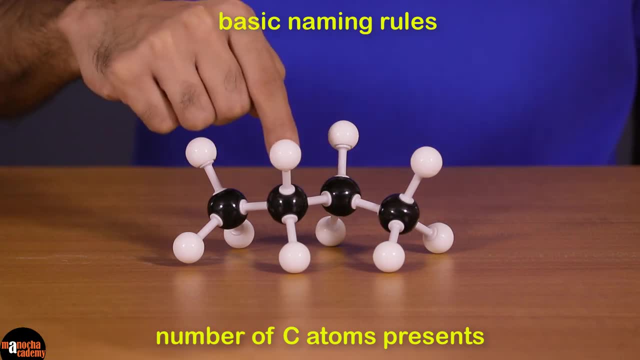 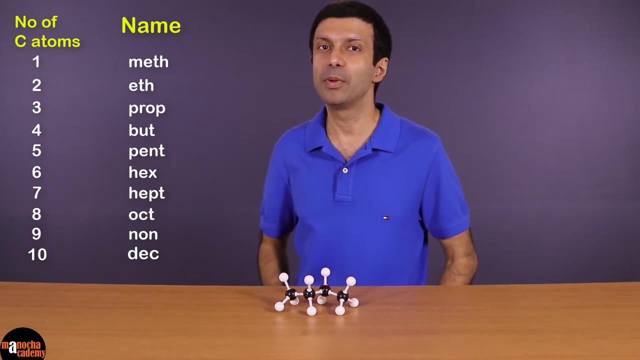 As you can see, we have a total of 4 carbon atoms. Now we need to look up this list. If the hydrocarbon contains 1 carbon atom, the name starts with meth. If it contains 2 carbon atoms, the name starts with eth, 3 carbon atoms, it starts with prop, And so on. I think. 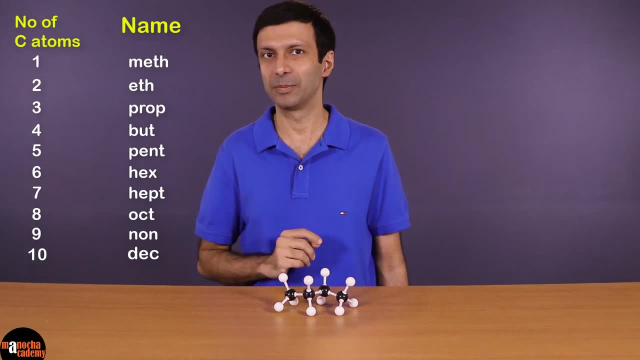 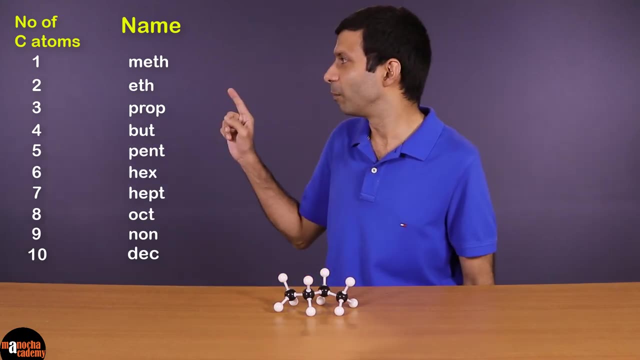 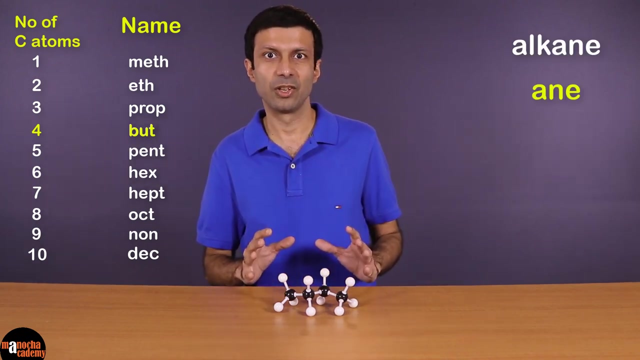 you have only till 10 carbon atoms in your syllabus. So now let's look at this compound. Since it has 4 carbon atoms, the name starts with but And the name ends with ane, because this is an alkane. So now, if we combine the two, 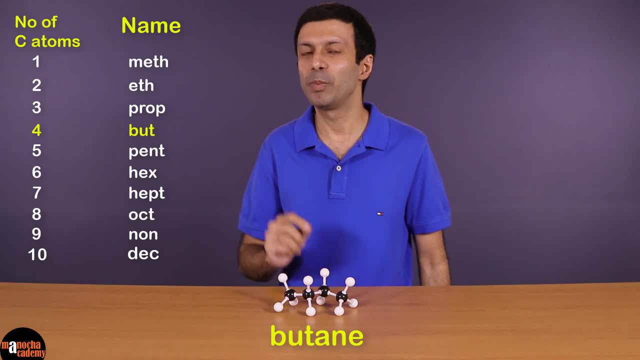 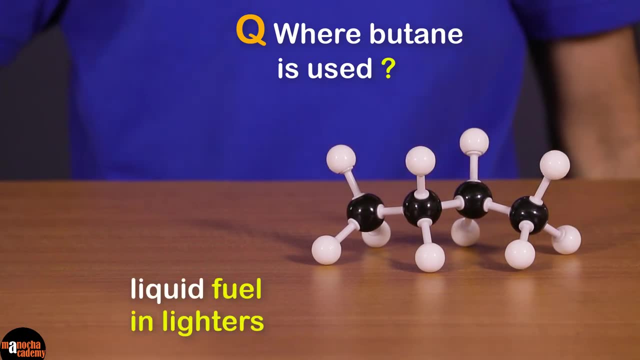 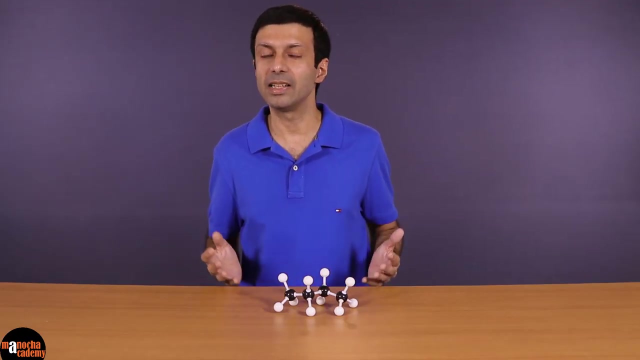 what's the name of this compound? That's right, it's going to be butane. Do you know where butane is used? That's right, it's the liquid fuel in lighters. And similarly, if we had an alkane containing only 2 carbon atoms, its name would have been: 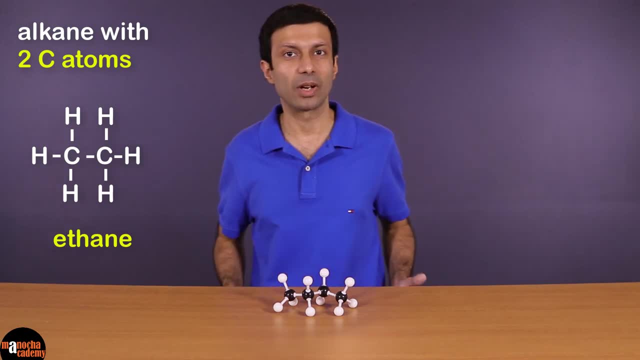 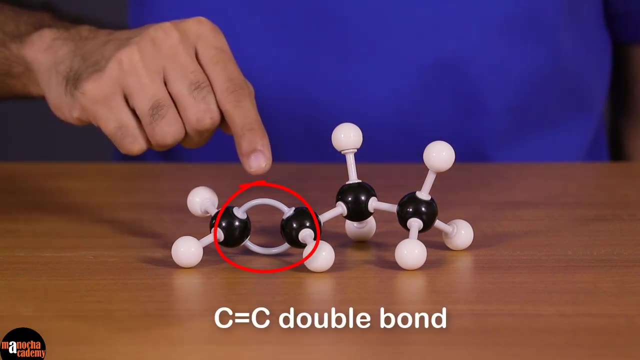 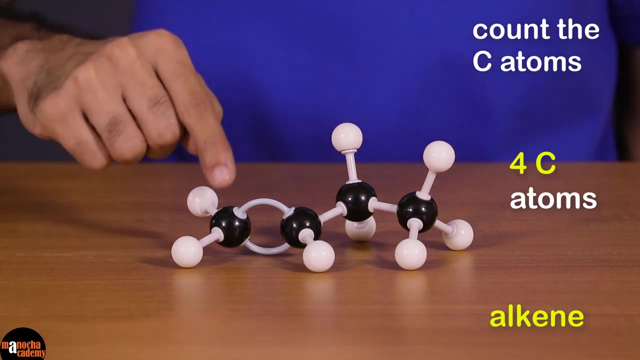 ethane. Now let's take a look at another hydrocarbon here. Since there is a carbon-carbon double bond, this is an alkene. Now let's count the number of carbon atoms. So here we have 1,, 2,, 3, 4 carbon atoms. So the name starts with, but 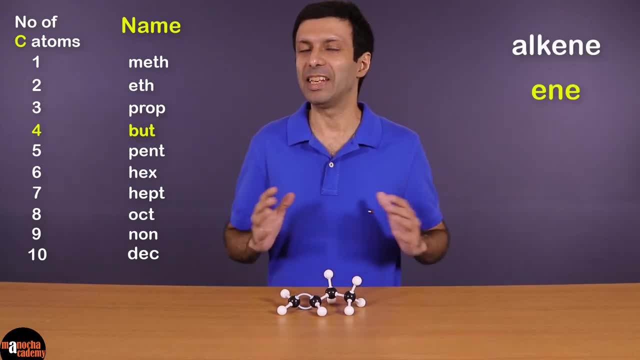 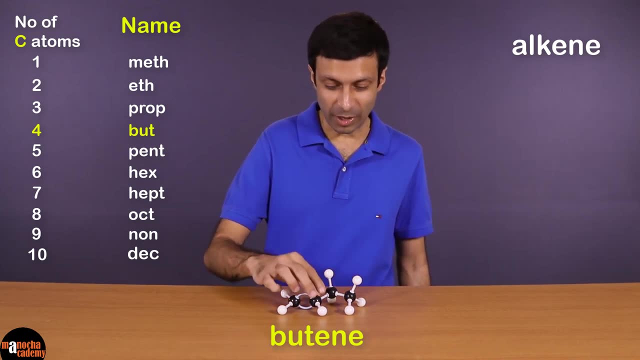 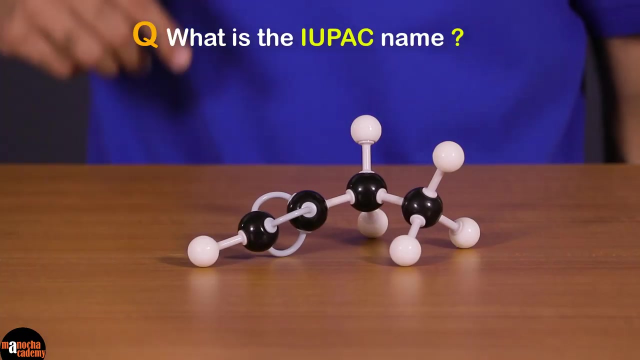 And since it's an alkene, the name ends with ene. So now, if we combine the two, the IUPAC name of this compound is butane. Now can you try to name the next compound here? What is the IUPAC name of this hydrocarbon? That's right. the correct answer is butyne. 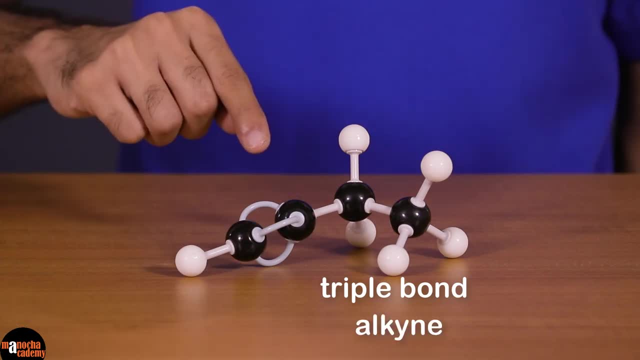 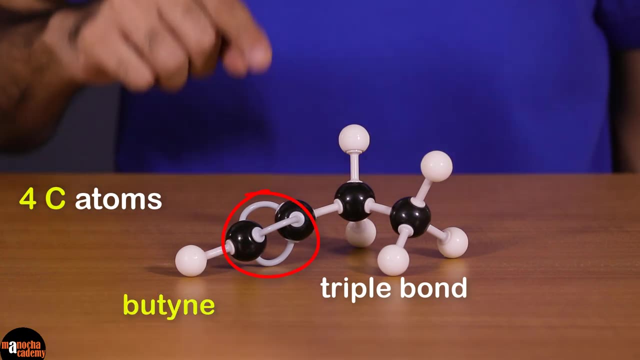 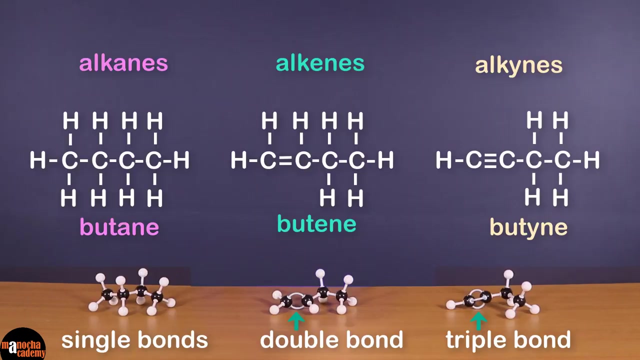 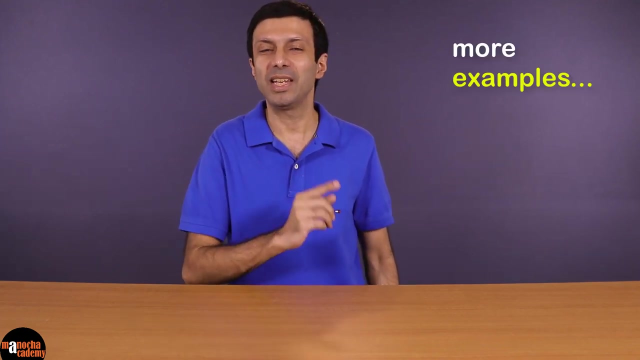 It has a triple bond, so it's an alkyne, So the name starts with but So the answer is going to be butyne. As we discussed, these compounds will be shown in your chemistry textbook like this: Now I'm going to show you some more examples, and you try to give me the IUPAC name, But 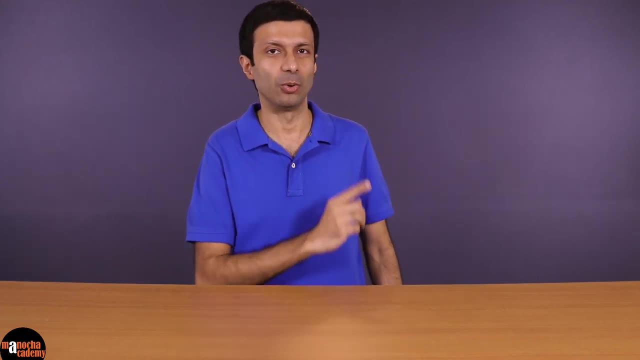 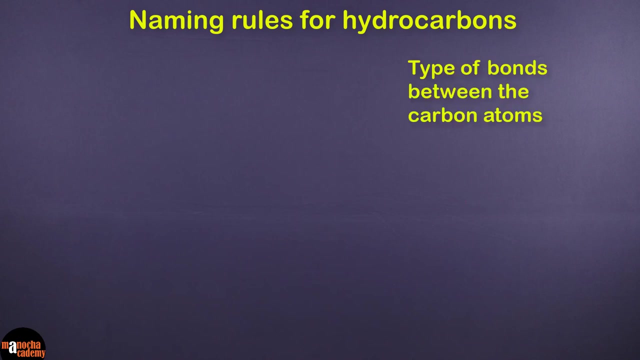 before that, let's do a quick recap of the naming rules. Let's revise the naming rules for hydrocarbons. Check the type of bond between the carbon atoms- Single, double or triple bond, Since this decides if it is an alkene, alkene or alkyne. Next, count the number of carbon atoms. 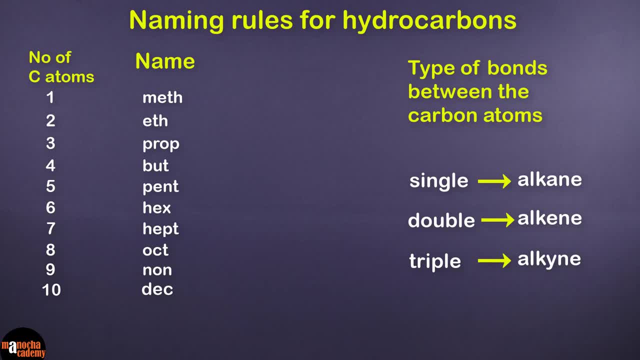 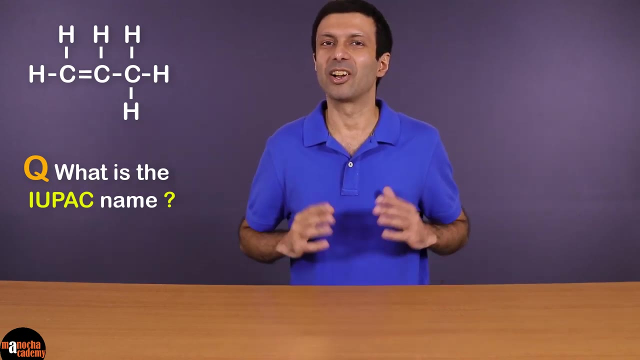 Using this list, decide the initial part of the name based on the number of carbon atoms. Join the initial part and the end to get the IUPAC name. What IUPAC name would you give to this compound? That's right? the correct answer is propene. 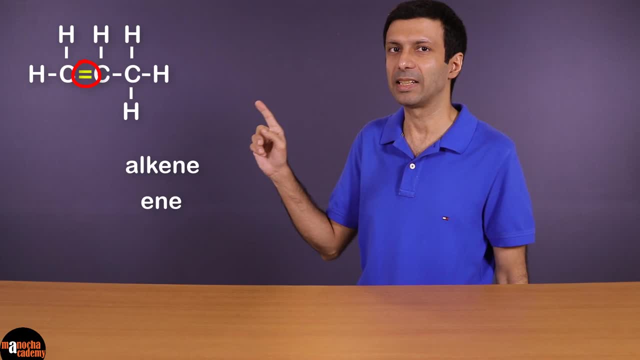 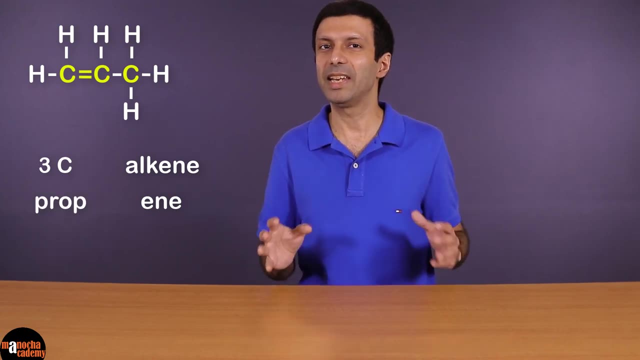 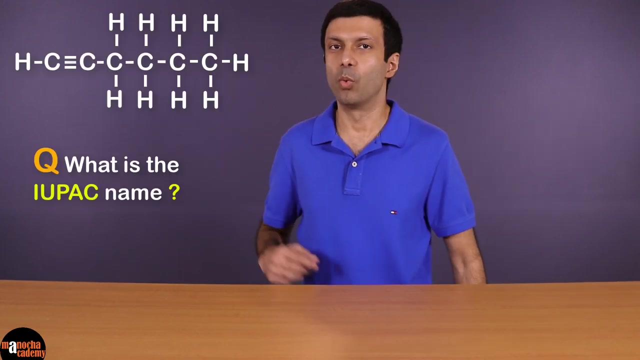 Can you see that there's a double bond there, So it's an alkene and there are three carbon atoms. So the name starts with prop, and combining the two we get the answer as propene. Now let's go ahead and try another compound. What will be the IUPAC name of this compound? 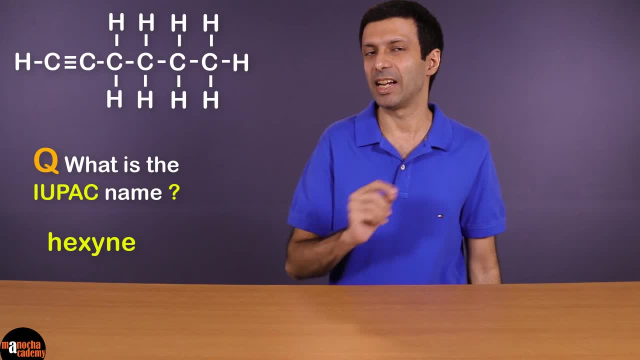 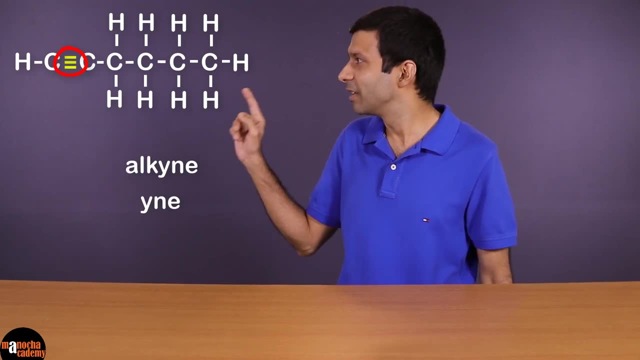 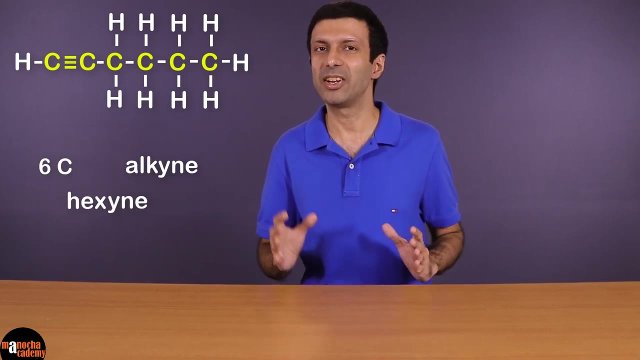 That's correct: hexine. Can you see the triple bond? So it's an alkyne, and there are six carbon atoms here, So the name starts with hex. Now, combining the two, we get the answer as hexine. As you can see, we can have many alkanes. 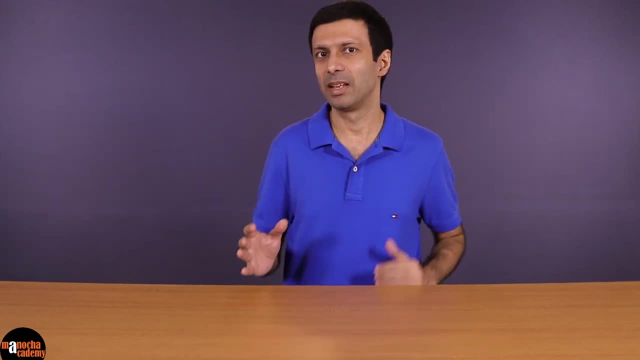 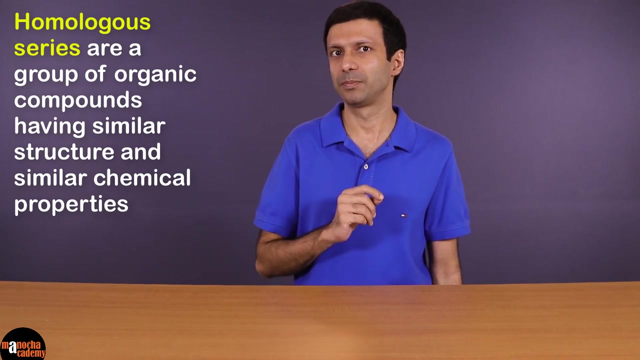 many alkanes and many alkynes. These are called homologous series of alkanes, alkenes and alkynes. Homologous series are a group of organic compounds having similar structure and similar chemical properties, For example methane, ethane, propane, butane. 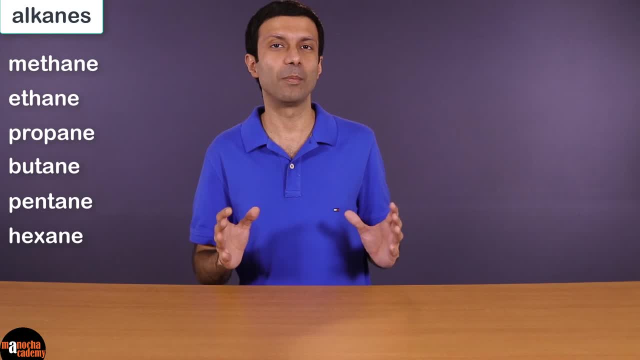 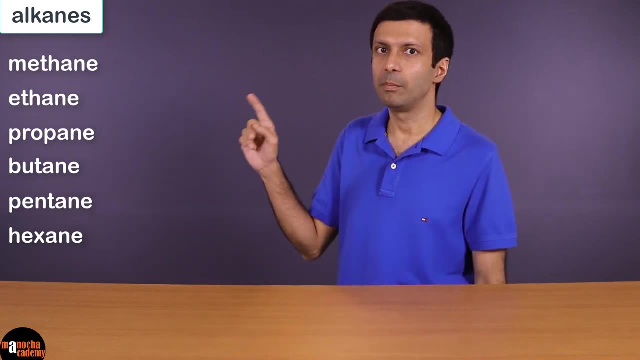 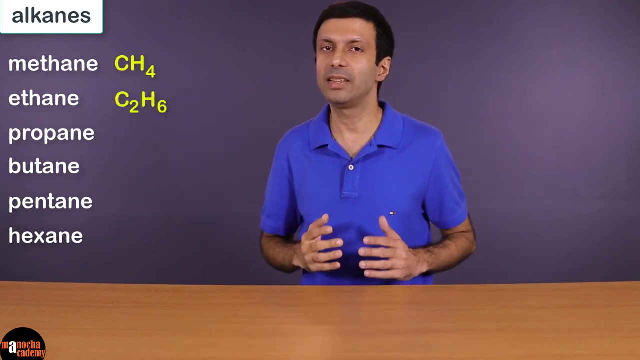 pentane, hexane and so on. These all belong to the homologous series of alkanes. Now, if you look at the molecular formula, methane is CH4 and ethane is C2H6.. So can you see that they differ by? 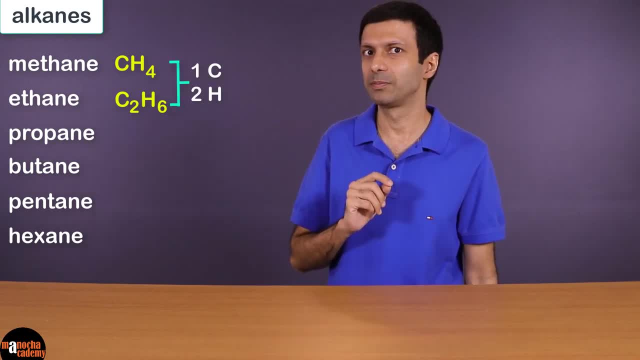 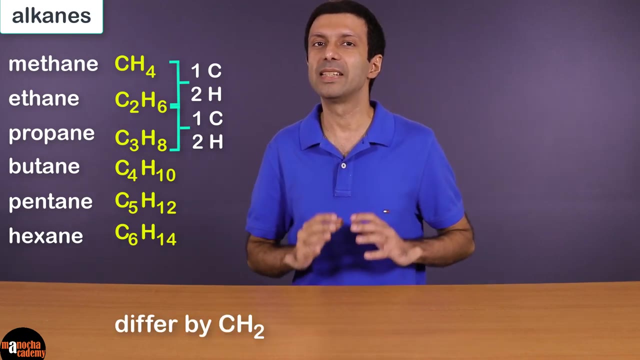 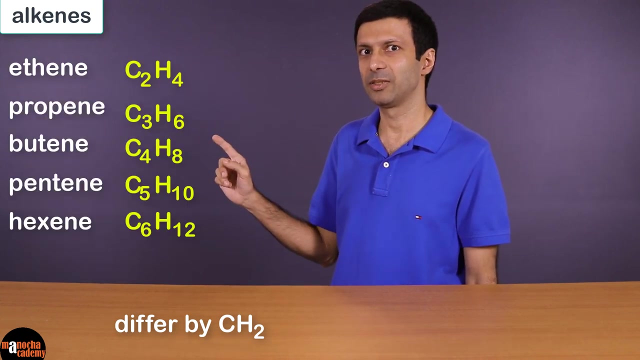 one carbon and two hydrogen atoms. Similarly, when you go from ethane to propane, again one carbon and two hydrogen atoms get added. So successive compounds in a homologous series differ by CH2.. And you'll notice this similar pattern for alkenes and alkynes. 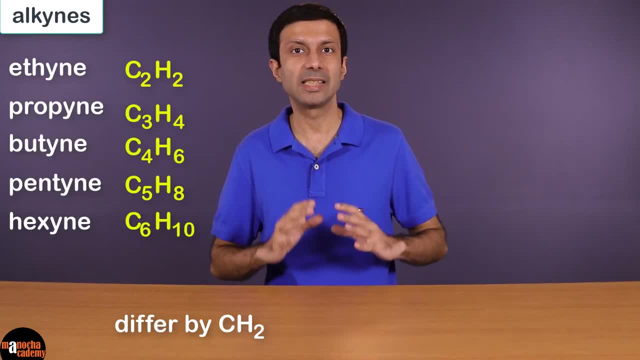 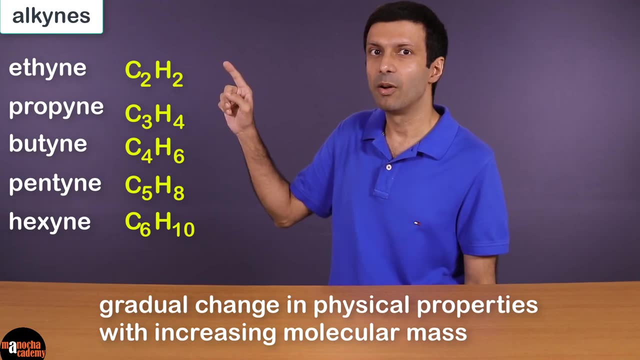 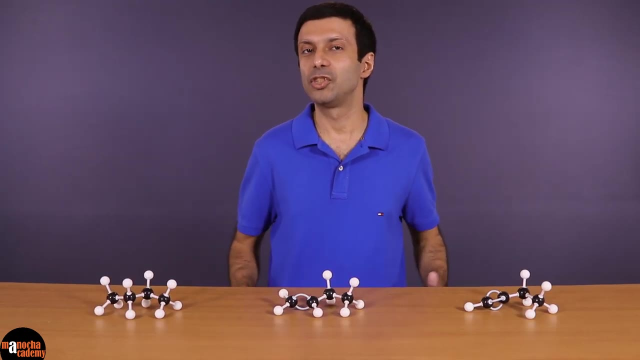 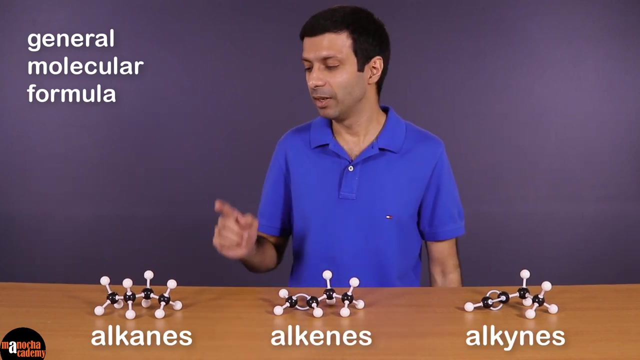 So homologous series are a group of compounds having similar chemical properties, but they see a gradual change in physical properties with increasing molecular mass, because every time CH2 gets added. Now let's look at the general molecular formula for alkanes, alkenes and alkynes. Let's start with. 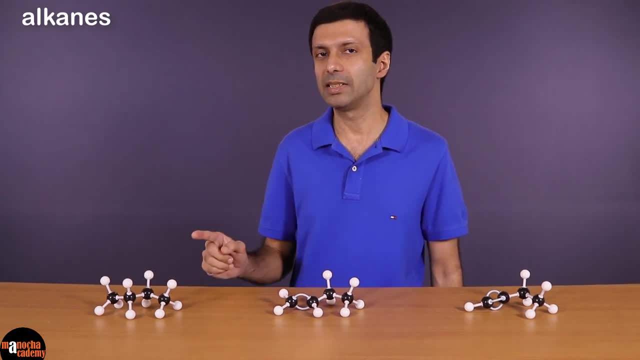 alkanes. The general formula for alkanes is CnH2n plus 2.. Now let's see if we can use this formula to quickly calculate the number of hydrogen atoms in butane. Butane has four carbon atoms, so n is 4. 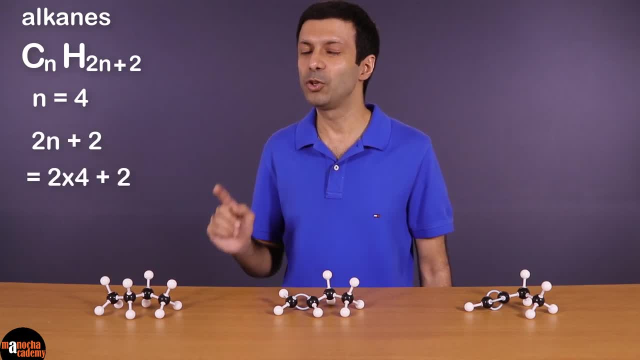 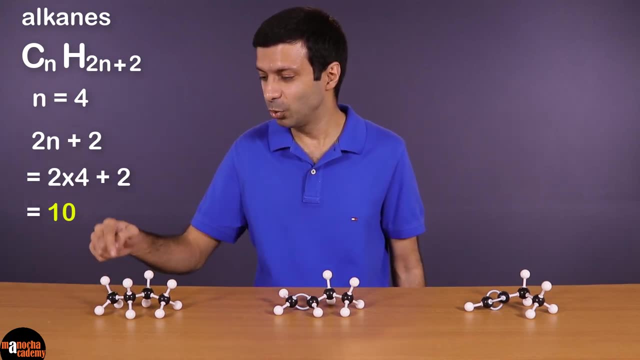 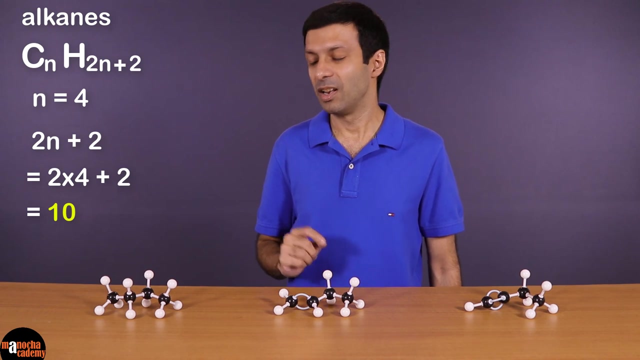 and the hydrogen atoms are going to be 2 into 4 plus 2, which is 10.. Now let's check Here we have 1,, 2,, 3,, 4,, 5,, 6,, 7,, 8, 9 and 10 hydrogen atoms. Now, using the 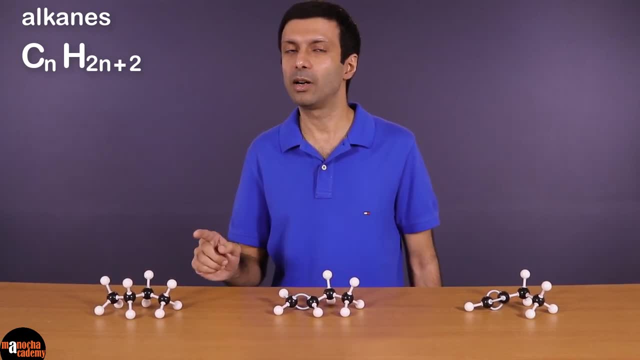 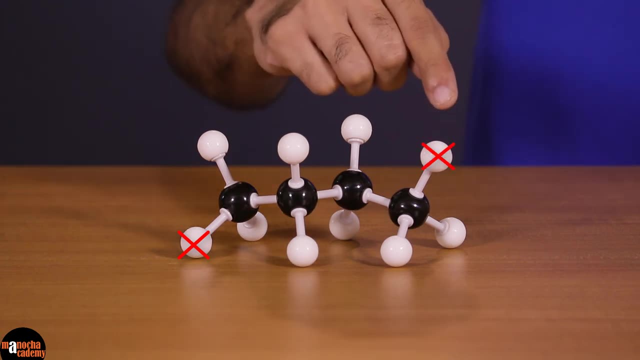 structure. let's see if we can understand why the formula is CnH2n plus 2.. If we ignore these two hydrogen atoms at the two ends for a moment, can you see that each carbon atom has two hydrogen atoms. So if the number of 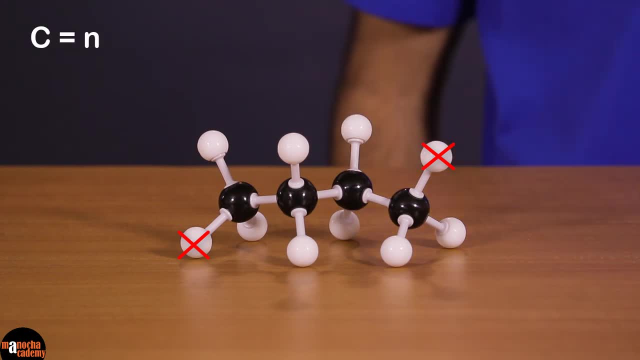 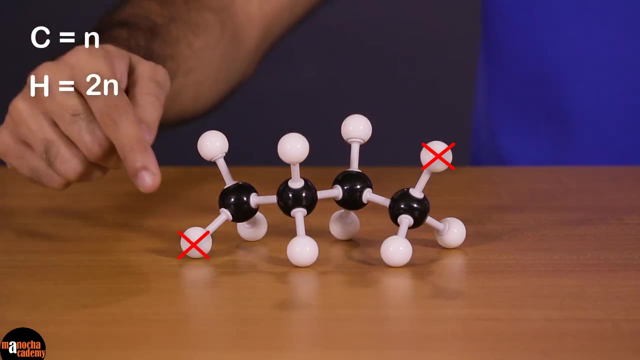 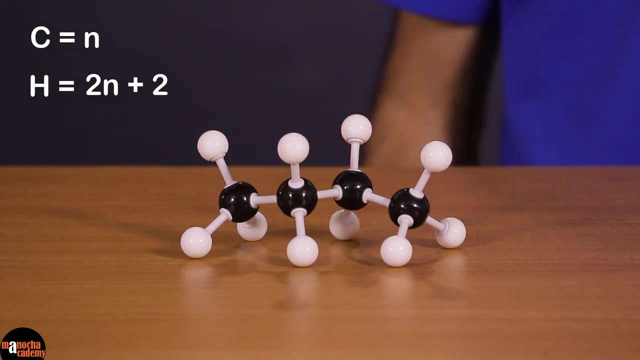 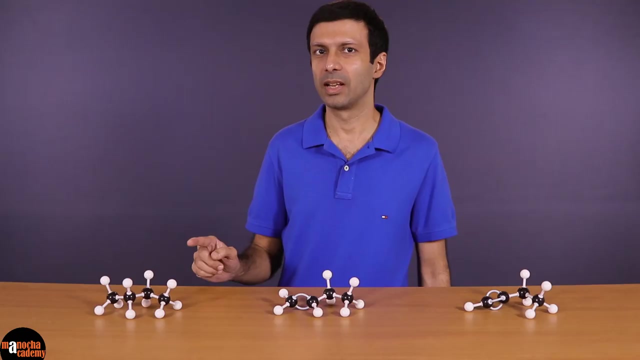 carbon atoms is n, the number of hydrogen atoms will be 2n. Now, each end carbon atom has one extra hydrogen in it, So the number of hydrogen atoms is 2n plus 2.. So that's how we get the general formula of the alkene: CnH2n plus 2.. Now 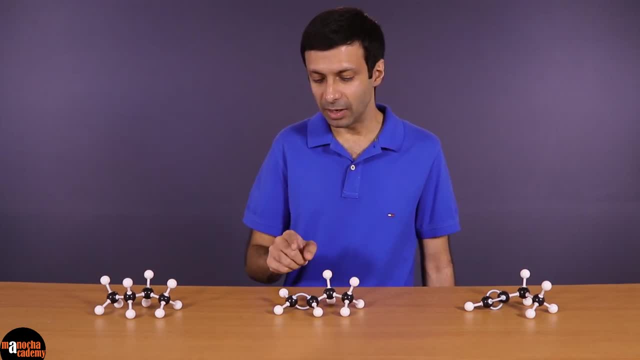 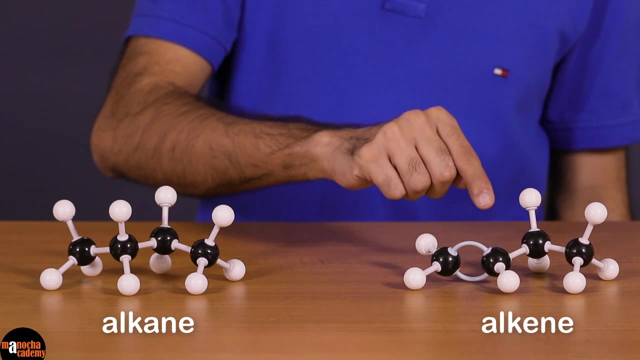 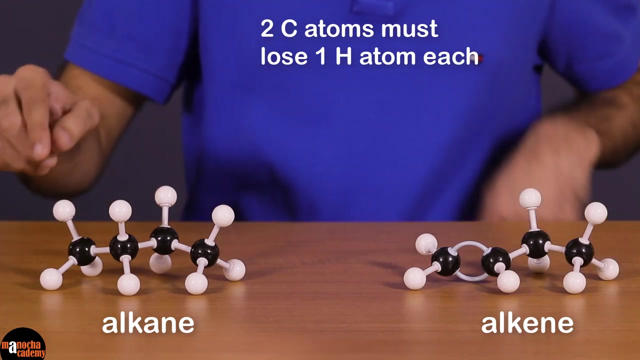 moving on to the alkenes, as you can see, there is a double bond between the two carbon atoms here. When going from an alkene to an alkene, the two carbon atoms forming a double bond must lose one hydrogen atom each. So I'm going. 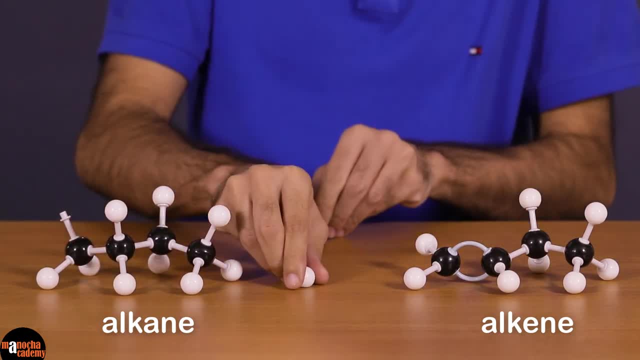 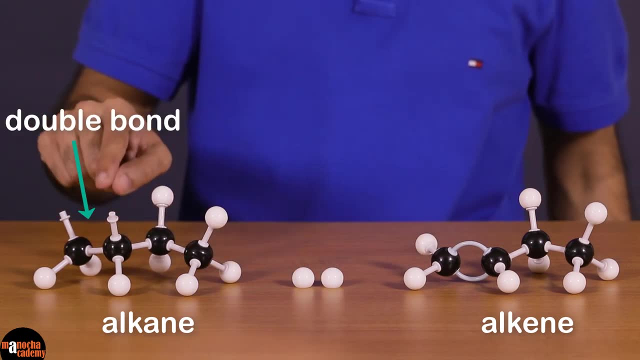 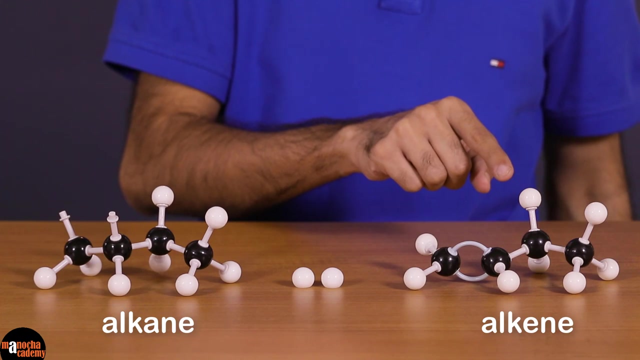 to remove these hydrogen atoms and the double bond gets formed here. So the molecule changes from this to this. So what's the general formula of alkene CnH2n plus 2?? So the hydrogen atoms are two less compared to the alkenes, The general. 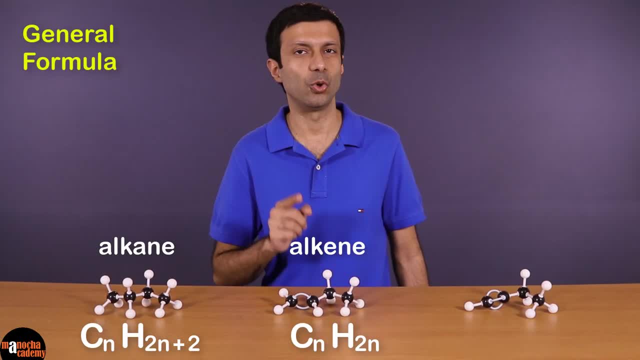 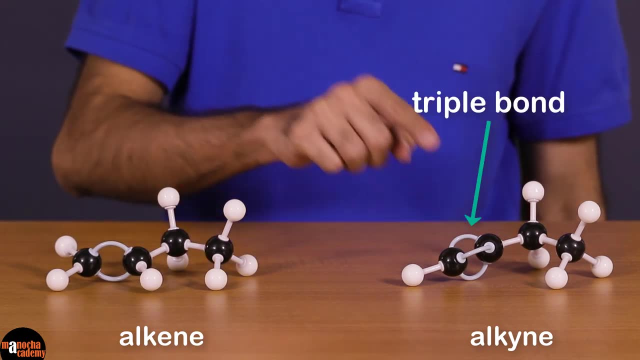 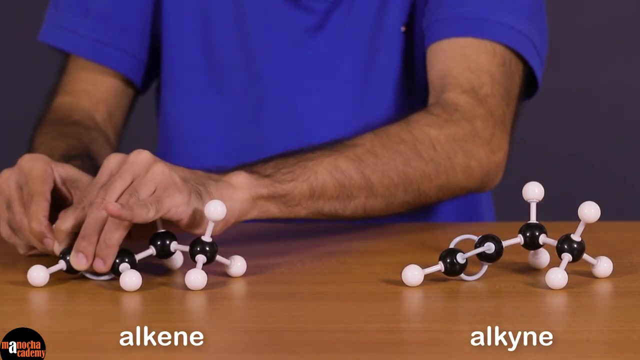 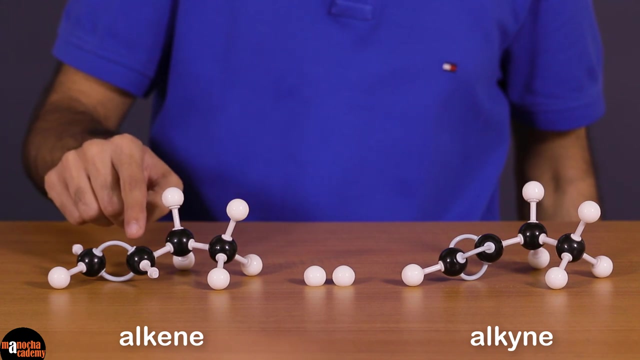 formula for alkenes is CnH2n. Now, moving on to the alkenes, the two carbon atoms forming the triple bond must lose one hydrogen atom each. So I'm going to remove these hydrogen atoms And these two carbon atoms will form the. 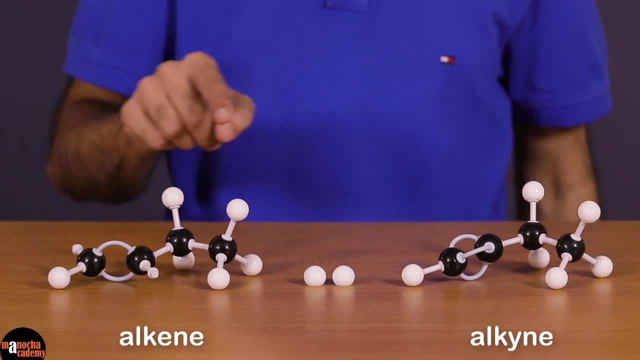 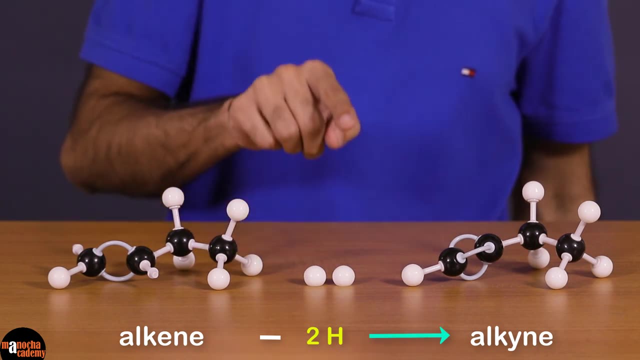 triple bond. So, as you can see, converting the double bond to the triple bond, two hydrogen atoms have been removed. So the hydrogen atoms in alkene is two less compared to the alkenes. So the general formula for alkene is CnH2n minus 2.. 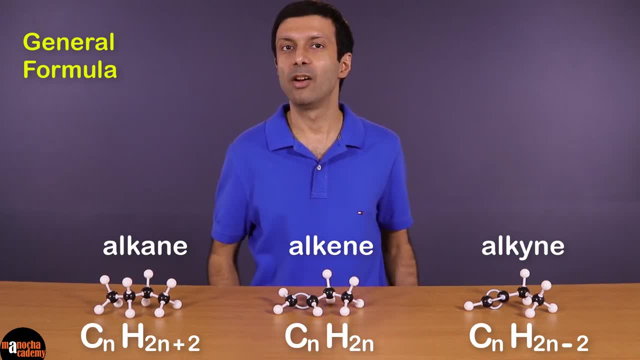 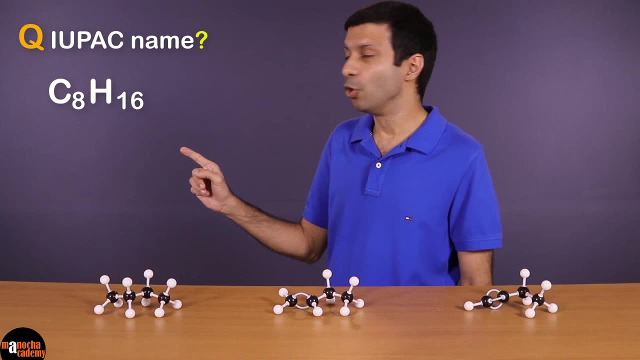 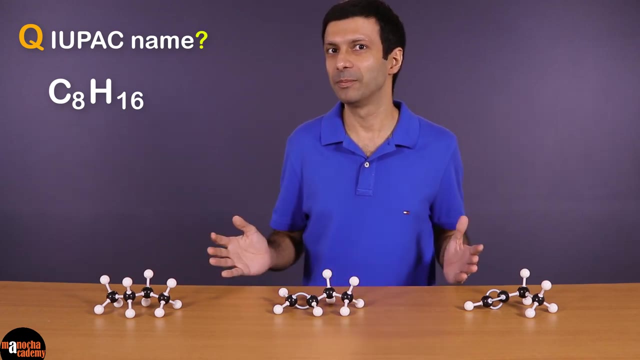 Now let's see how we can apply this formulae for naming. Can you name this compound C8H16?? Note that we are only given the molecular formula, not its structure. So what's the IUPAC name going to be? That's right, the name of this. 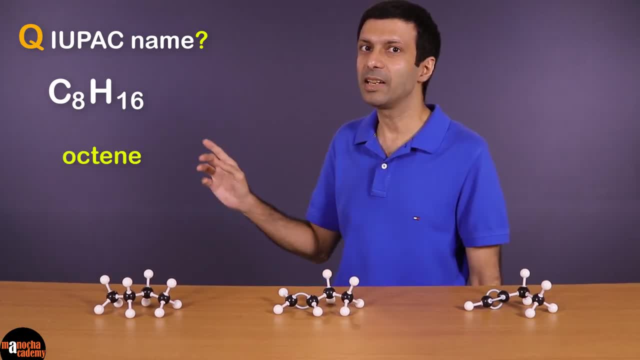 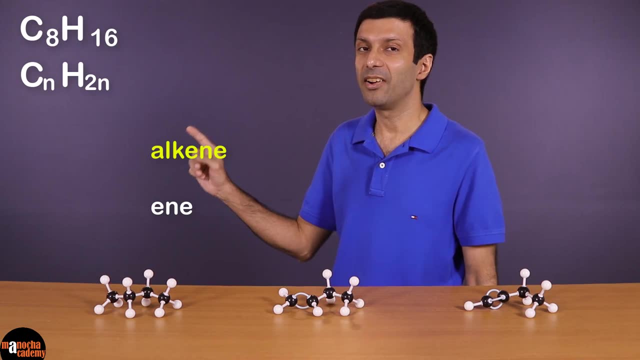 compound is octene. Can you see that? it fits into the pattern of CnH2n, So it's an alkene and there are eight carbon atoms. So the name must start with oct, And combining the two we get the name.